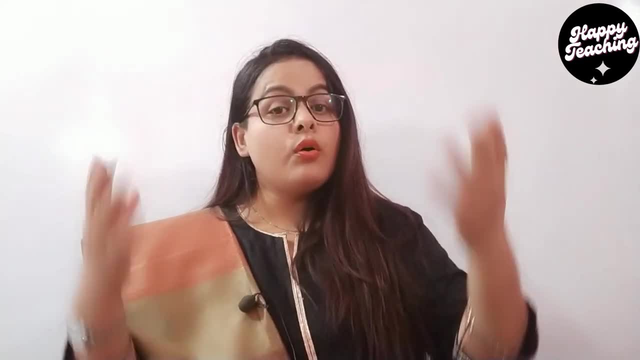 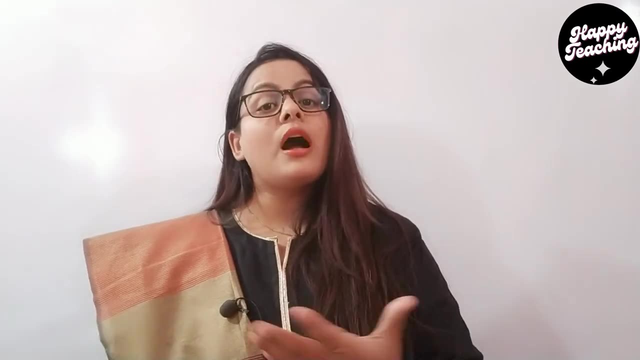 to the students. but the interviewer will going to see your overall personalities, okay, your body language, your facial expression and so many things: how well you manage your classroom, how well you manage your students, how well you reply to your students queries. okay, so these are the things you 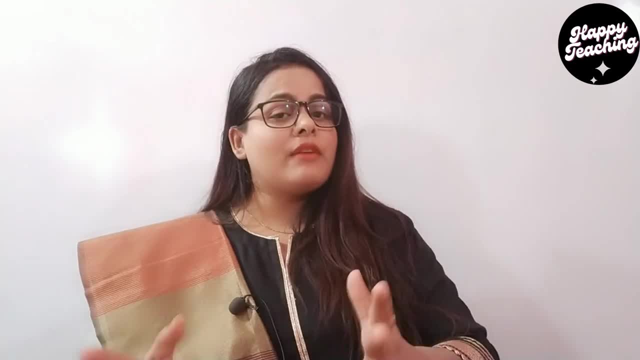 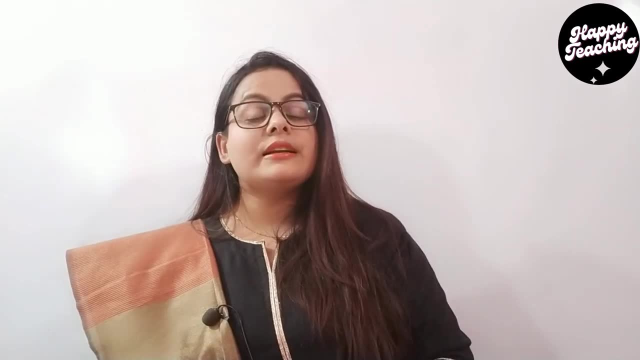 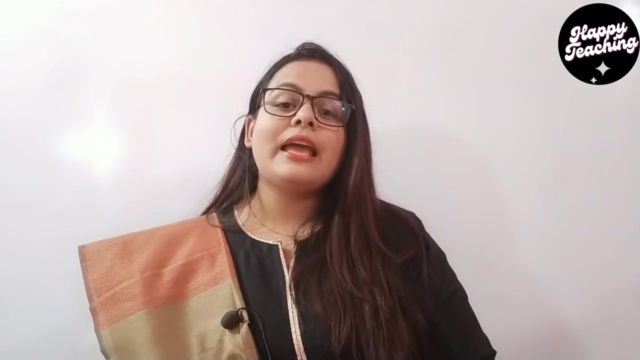 should prepare before your interview, and I know that you have a very good command in your subject, but somehow you fail to prove yourself Here. in this video, I am sharing few sentences which are really helpful for you, Which you can use at the time of your demo teaching. okay, and one more thing. I have many videos like this. if you're interested to check, you can check in the description box. 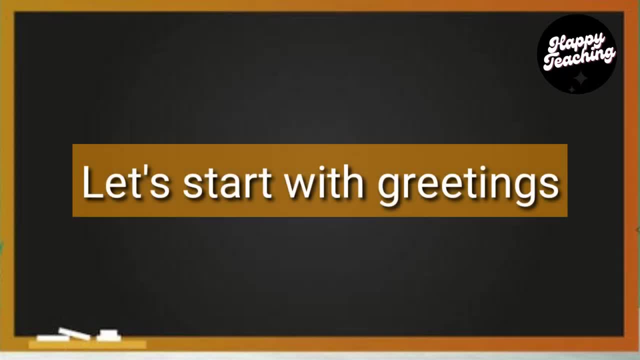 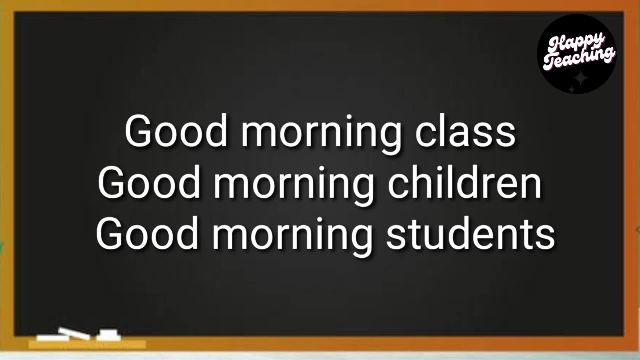 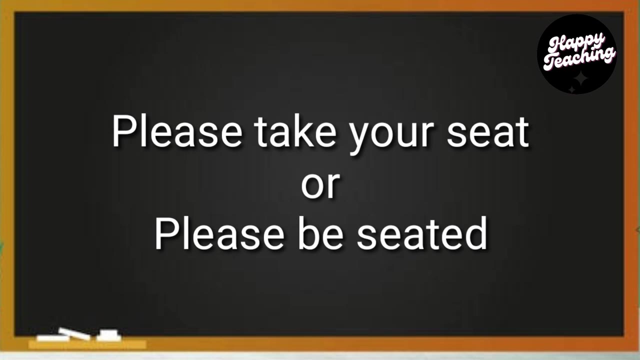 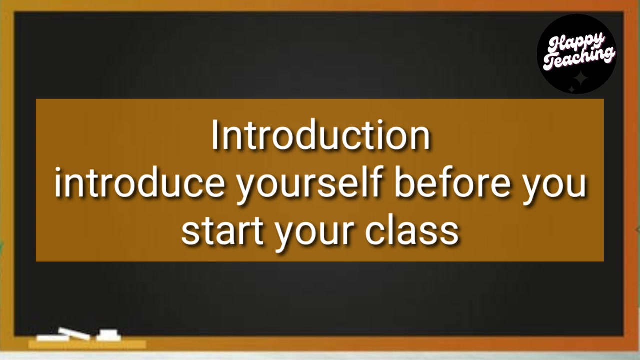 So, without further delay, let's start. Let's start with greetings. Good morning class, Good morning children, or good morning students. How are you all Nice to meet you. Please take your seat. or you can say: please be seated after that introduction. introduce yourself before you start your class, like so, all right, children. 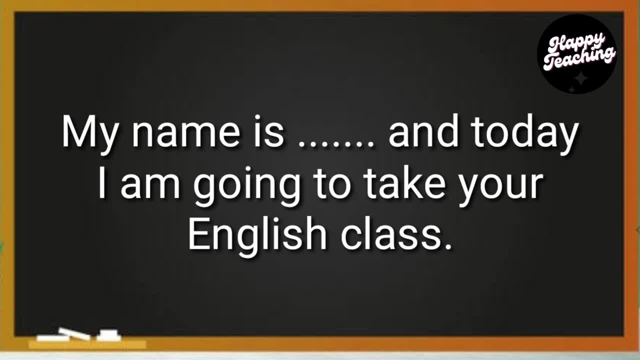 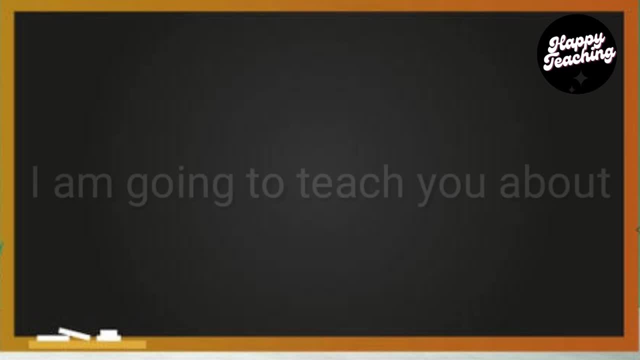 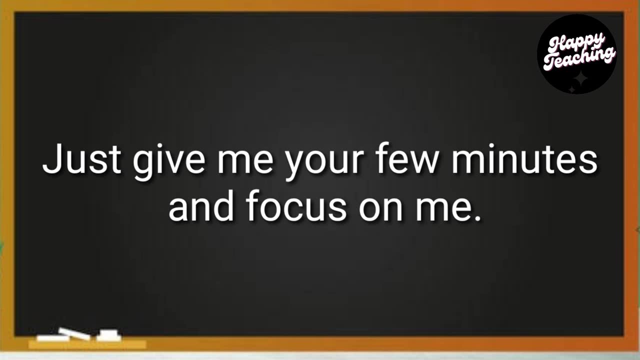 my name is dash and today i am going to take your english class, or you can say i am going to teach you about the topic which you are going to teach. just give me a few minutes and focus on me. just give me a few minutes and focus on me. feel comfortable if you want to talk, feel comfortable. 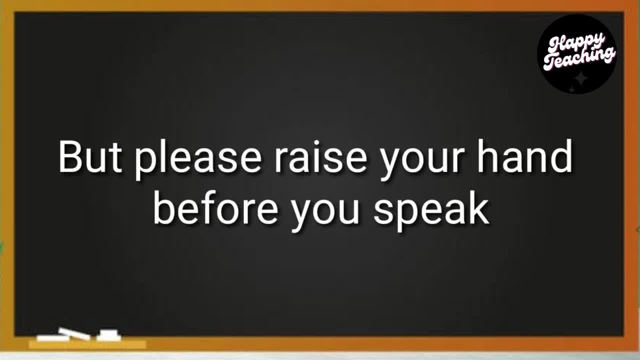 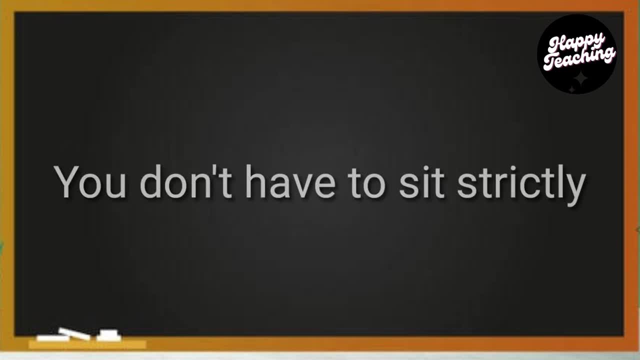 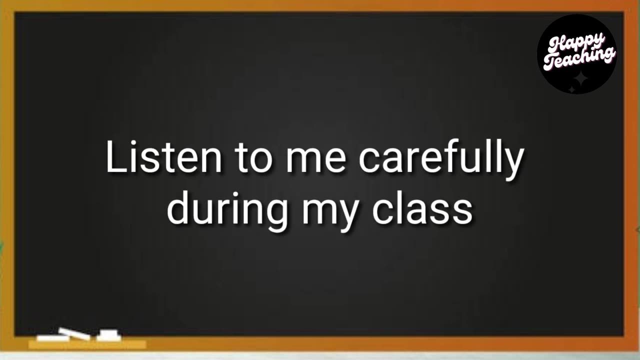 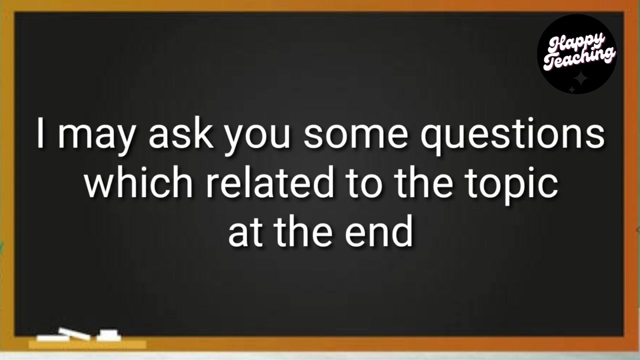 if you want to talk, but please raise your hand before you speak. but please raise your hand before you speak. you don't have to sit strictly, so make yourself comfortable. so make yourself comfortable. listen to me carefully during my class. listen to me carefully during my class. i may ask you some questions which related to the topic at the end. 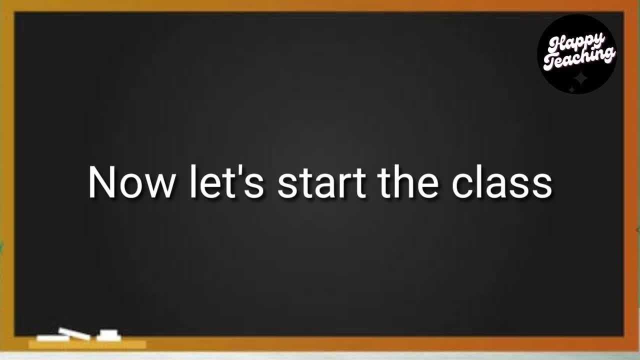 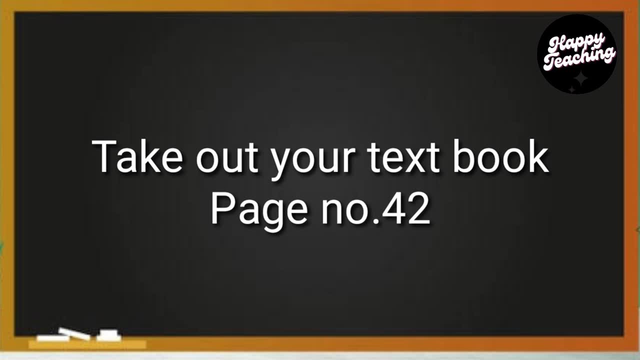 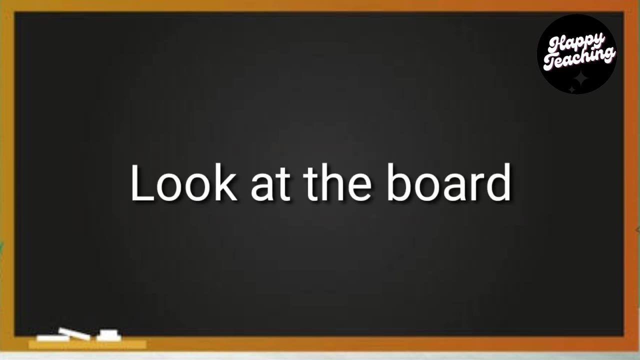 so can we go ahead? or you can say: now let's start the class. take out your textbook. take out your textbook, page number 42. now, introduction of the topic. look at the board. look at the board. i'm going to explain this topic. i'm going to explain this topic. 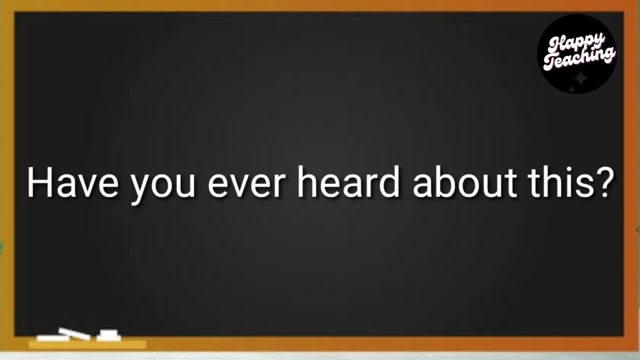 have you ever heard about this? have you ever heard about this? what do you know about it? what do you know about it? or have a guest? students have a guest children. that's correct, outstanding. it's good to see all your efforts and knowledge if you have a guest. 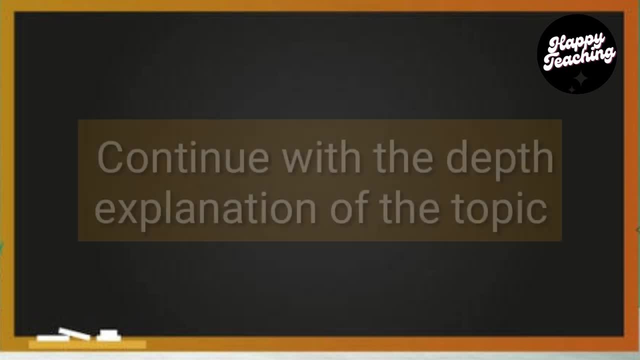 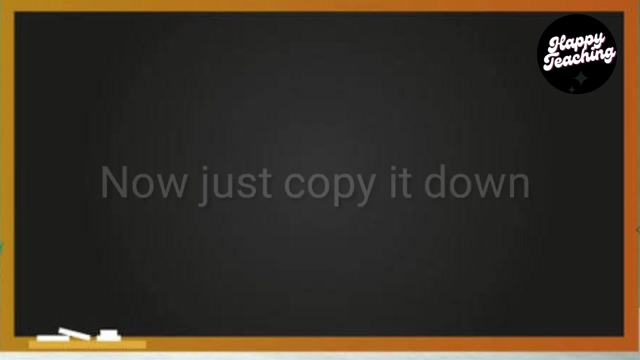 it's good to see all your efforts and knowledge and after this, continue with the depth explanation of the topic. for the important line you can say: underline this line with pencil: can you speak louder? can you please speak louder now? just copy it down, class. lastly, conclusion revise. 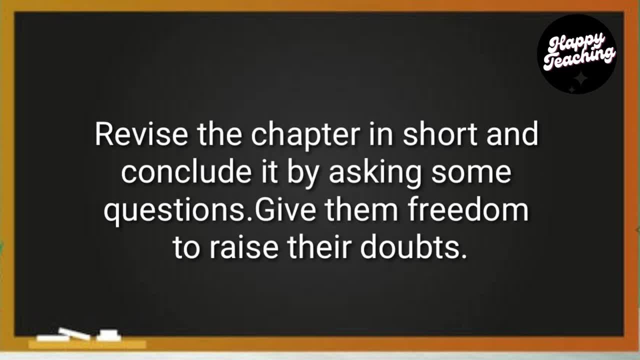 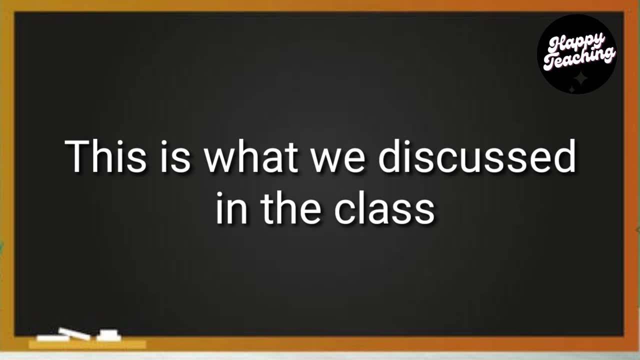 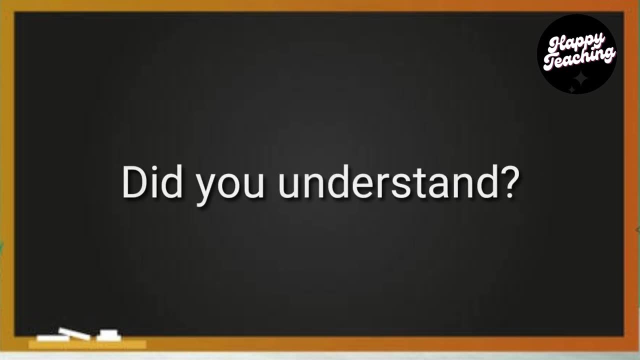 the chapter in short and conclude it by asking some questions. give them freedom to raise the doubt. this is what we discuss in the class. student, this is what we discuss in the class. is there is any doubt? is there is any doubt? did you understand? hope the topic is clear to everyone. 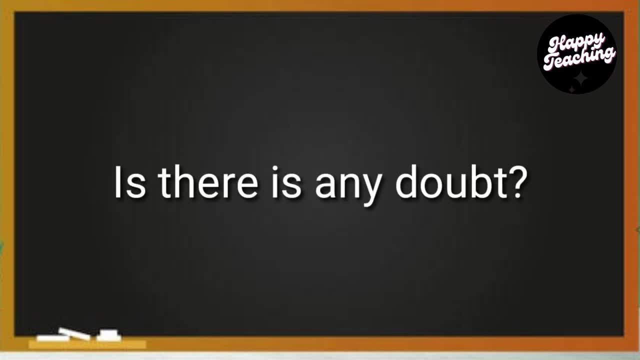 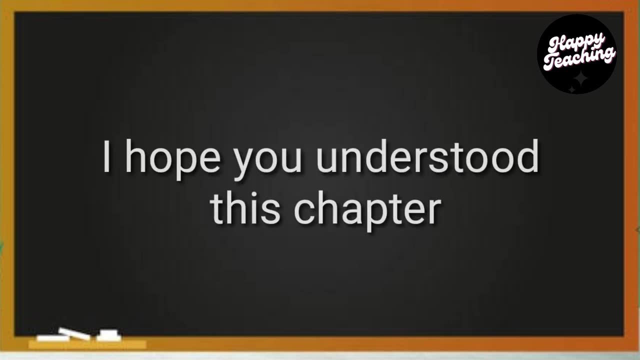 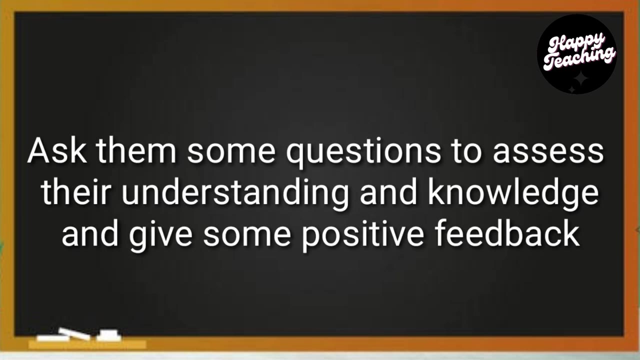 hope the topic is clear to everyone. is there is any doubt? is there is any doubt, please feel free to ask your doubt. i hope you have understood this chapter. hope i'm clear to you Now. ask them some questions to assess their understanding and knowledge and give some positive feedback for this. 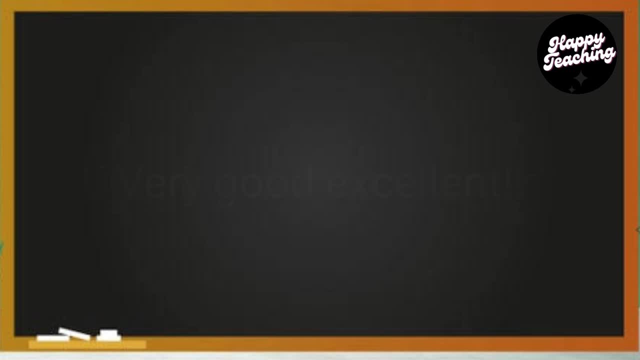 Who knows the answer? Very good, Excellent, Good try. Yes, that's right. Come out and write it on the board. Speak one at a time, please. Speak one at a time, please, Not bad, Hmm, it's different. 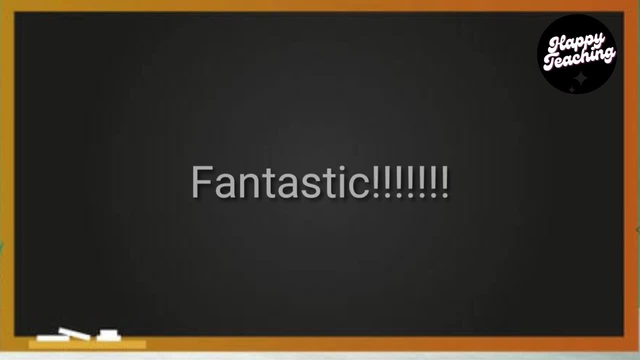 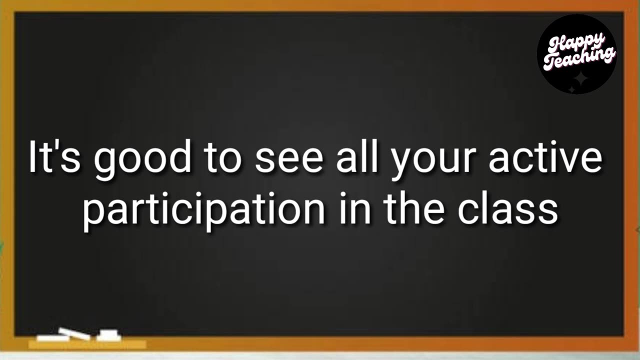 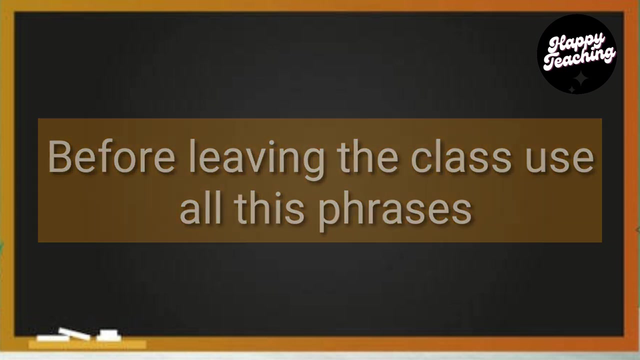 Good work, Keep going. Fantastic, Superb. It's good to see all your active participation in the class. It's good to see all your active participation in the class. Now, before leaving the class, you can use all these phrases: Thank you, everyone. 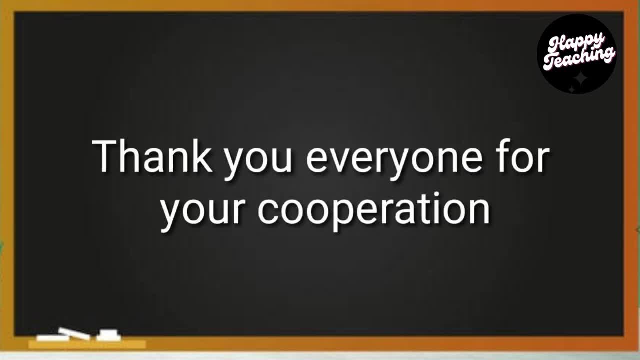 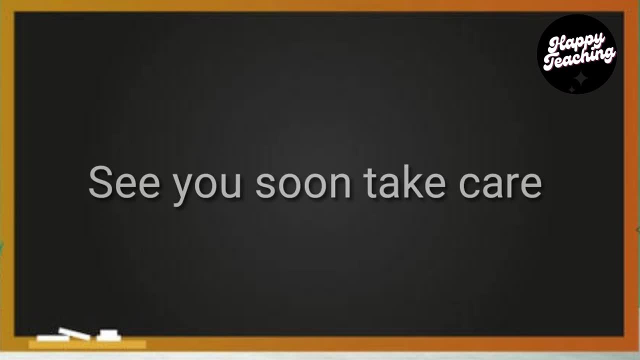 Thank you for paying attention. Thank you everyone for your cooperation. Thanks for your patience. Thank you very much. See you soon. Take care, Have a nice day. So that's all about this video. I really hope that you found this video helpful for you.